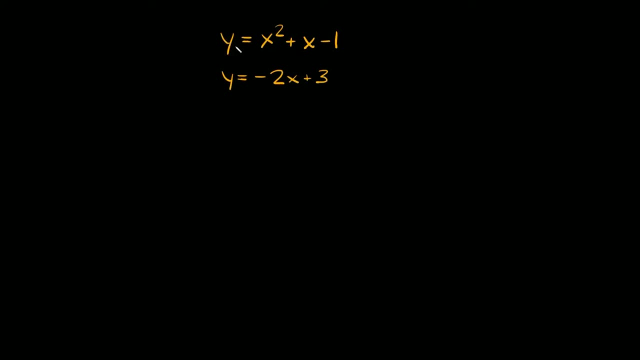 an example of each one. So let's do this one first. So this one is: y is equal to x squared plus x minus one, and y is equal to negative two x plus three. So, as you can see, it's saying that y is equal to all this crap over here, and y is also equal to all this crap over here. So the 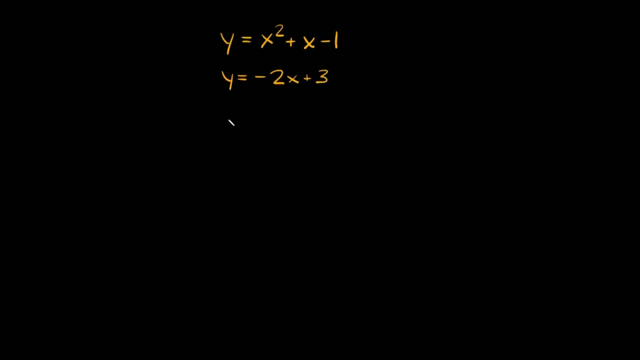 first thing we can do is set this crap equal to this crap right here. So that's what we're going to do. We're going to say x squared plus or sorry, plus x minus one is equal to this one over here. negative two x plus three. Okay, now the second step is just getting all your terms on one side. 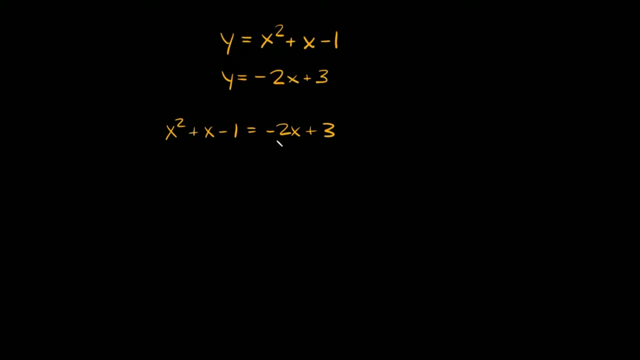 and the reason we have to do that is because we're going to have to factor. Okay, so the first thing I'm going to do here is add two x to both sides, and then I'm also going to add or subtract three from this. So then on this side, these terms cancel out right, they just go to zero. and then on this side, we're 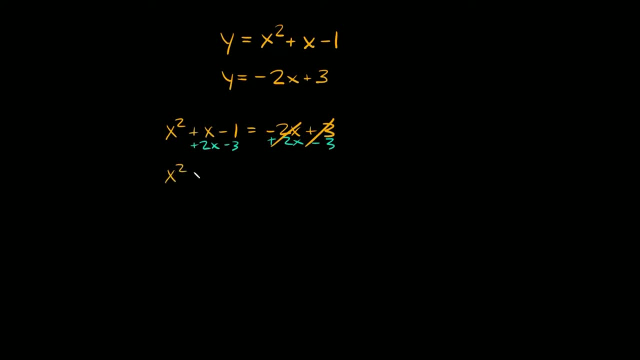 going to have x squared plus three. x minus four is equal to zero, right, since we don't have anything on that side anymore. Okay, so this is what we're going to have to factor, So we have again x squared plus three, x minus four. Okay, so we're going to factor this. now we have an x squared here, so we 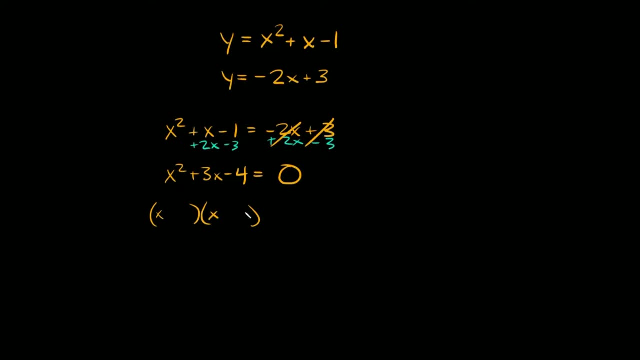 can break that down into x times x and then to figure out the two x squared plus three x minus two numbers that go right here, they have to multiply to negative four. Okay, they have to multiply to negative four. so two numbers that multiply to negative four. but they have to add up. 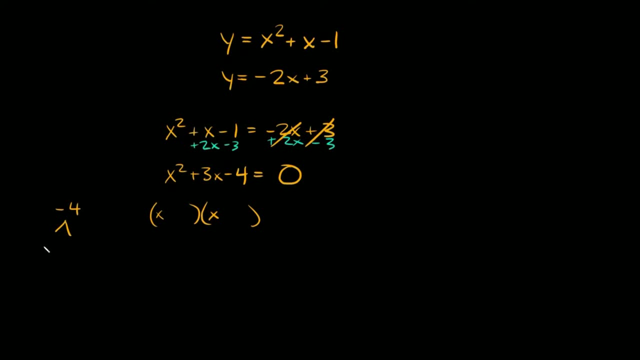 to positive three, the middle number. Okay, so in this case we would have to use a positive four and a negative one, right? because four times negative one is equal to negative four, and four plus negative one is equal to positive three. So positive four and negative one, and again this is. 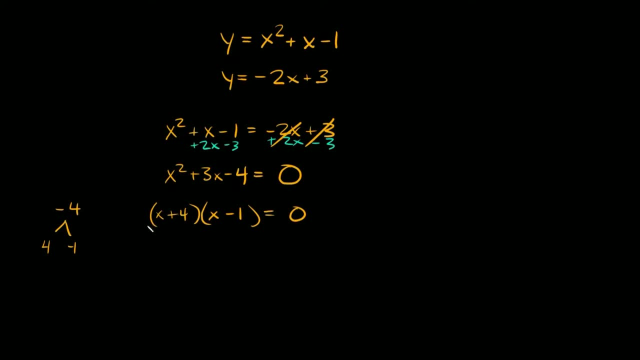 all equal to zero. Okay, and then the last thing we have to do here is we're going to have to add: here is just set each of our parentheses equal to zero. So we have: x plus four is equal to zero, and x minus one is equal to zero, right? So then, on this top one, our answer would be: x is equal to. 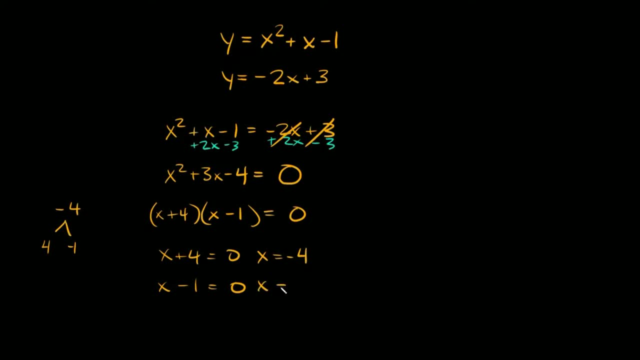 negative four, and then, on this bottom one, our answer would be: x is equal to positive one. Okay, so you get two answers, right? basically one for each set of parentheses. Okay, so, since we got two answers for x, we're going to basically get two answers for y, and the way that we find y now is just by plugging these back into one of these. 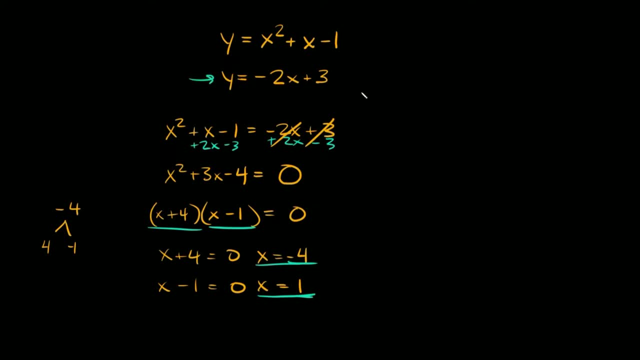 original equations and I'm going to pick this one right here because that one looks like it's a lot easier to work with. Okay, so this one is, and I'll write it over here: y is equal to negative two x plus three. Okay, so let's plug in our first x term right here, so we're going to get: y is equal to: 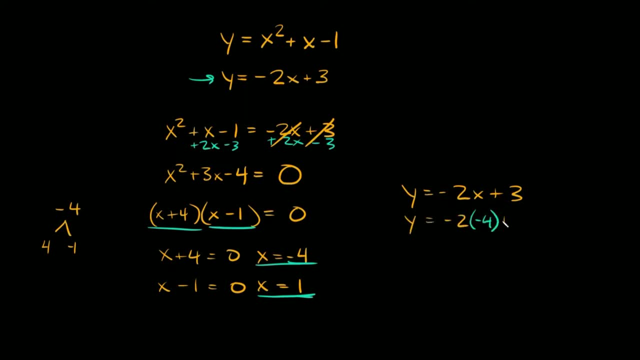 negative two times negative. four plus three, and that's equal to- let's see- negative two times negative. four is positive eight, so eight plus three is eleven. Okay, and then for our other one we're going to get, y is equal to negative two times positive. one plus three. Okay, so negative two times one is negative two and negative two plus 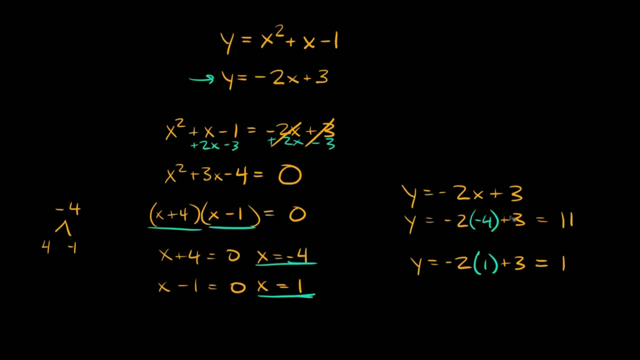 three is equal to positive one. Okay, and I'm going to move these down just to kind of match them up a little bit more clearly. So first we plugged in x is equal to negative four, and we got y is equal to eleven. Okay, so that's our first answer, or first pair. 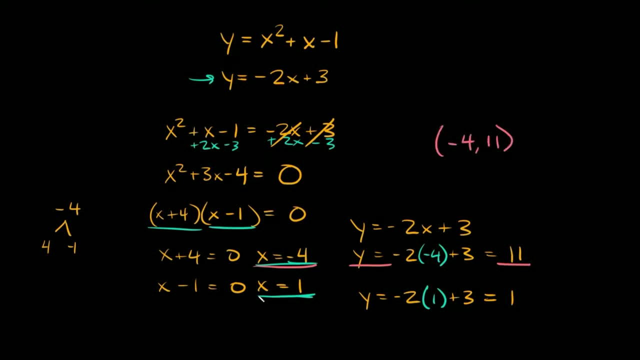 Negative four, eleven. and then the second one we did was: x is equal to one. and then we got: y is equal to one also. All right, so that's our second solution, or our second pair, so that one's at one comma one. Okay, so those are your two solutions to this system of equations. Okay, here's the next. 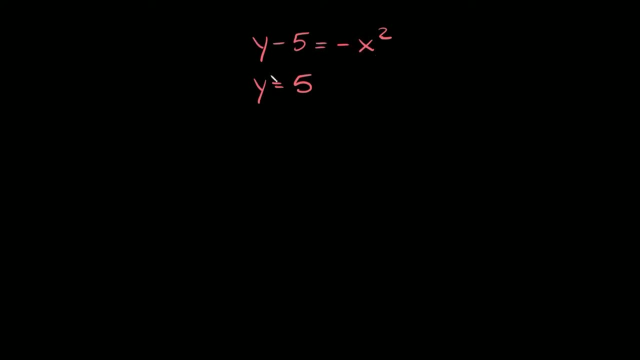 one. so we have: y minus five is equal to negative, x squared and y is equal to five. Okay, so one thing we can do here is well, the second equation. it's basically two times negative, two times, telling us exactly what y is equal to right: it's equal to five, So we can just plug in a five. 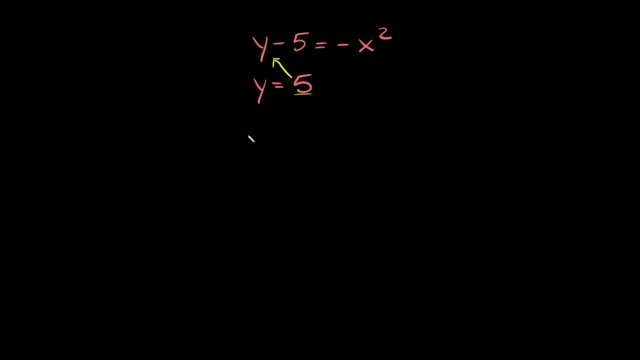 for y, right there? Okay, so then we'll plug in the five for y. so we're gonna get: five minus five is equal to negative x squared. Okay, five minus five is zero, so zero is equal to negative x squared. Okay, now to get rid of the negative sign, we can divide both sides by negative. 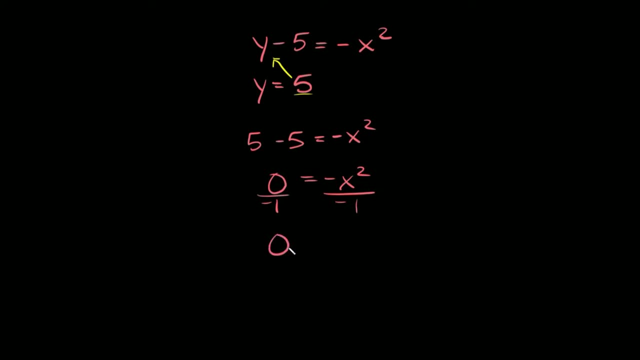 one. So zero divided by negative one is zero. so we get zero is equal to. then those basically cancel out. so we get x squared right. So we get x squared is equal to zero. Now the only number we could possibly plug in for x right here would be zero right, because zero squared is equal to zero. 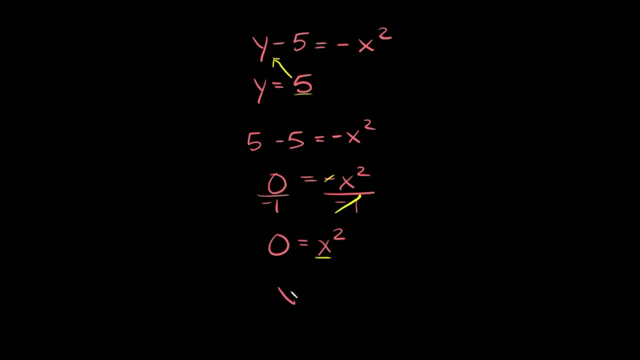 So here we have one solution for x. we have x is equal to zero. Okay, so we know what our x coordinate is, and then we can plug it in back into one of these equations over here. but if you notice something, it already tells us exactly what y is equal to, right? it says y is equal to five. 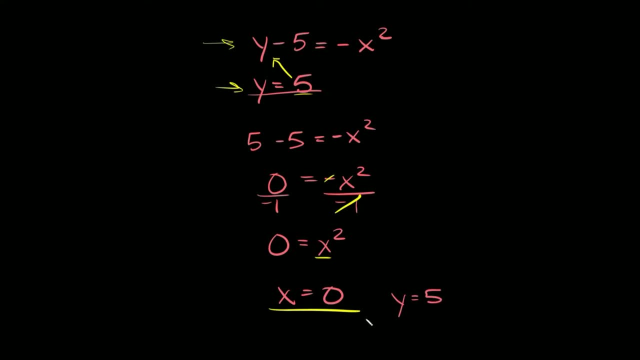 So we know that y is equal. Okay, so then our answer or solution, our ordered pair, would be zero comma five, right? So then this problem would only have one solution, Okay. and lastly, here we have: y is equal to negative x plus seven, and y is equal to negative x squared minus two, x minus one. Okay, so again, it's saying that. 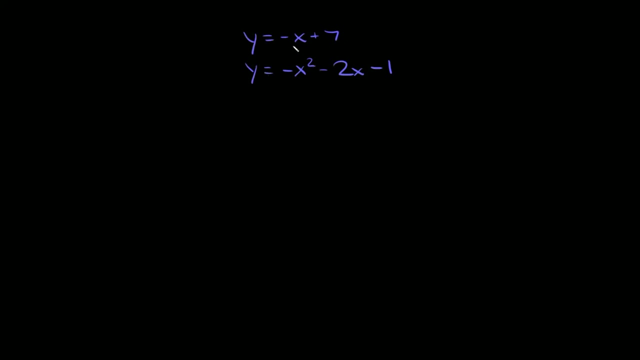 y is equal to all this over here, and y is equal to all this over here. So we can just set all of this equal to all of this. All right, so that's what we're going to do. So we're going to say: negative x plus seven is equal to negative x squared minus two. x minus one. Okay, and then you. 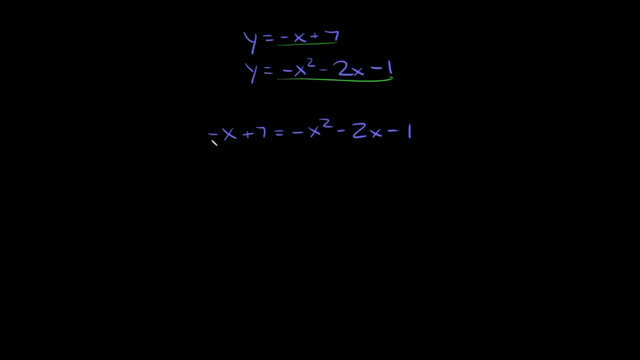 just want to again get everything on one side, So we'll move it all to the right. So here we're going to add x and we're going to subtract seven, right? So then on this side we're going to add x and then subtract seven. Okay, so then over here, those cancel out. this whole side goes to zero. 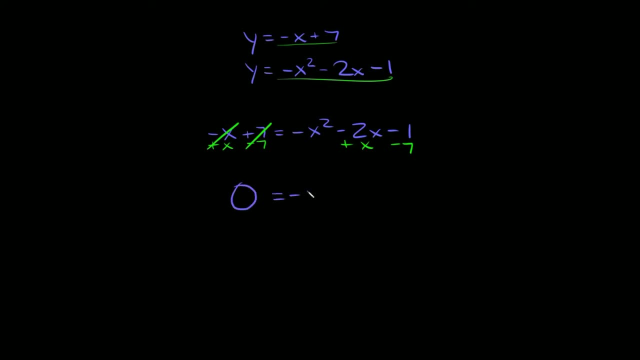 All right, so we're going to get: zero is equal to negative x squared minus minus x minus eight. Okay, now I don't like this negative x squared over here. So what I'm going to do is I'm going to divide this whole side by negative one, and again what we do to one side. 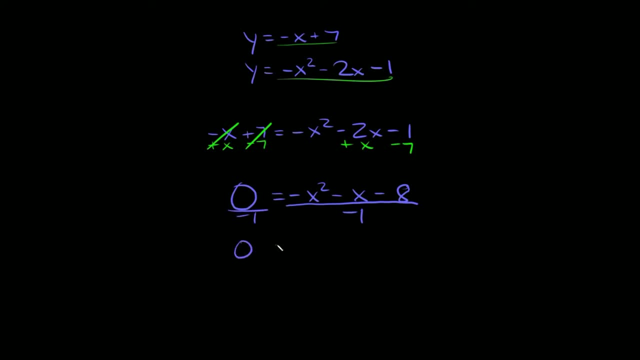 we do to the other, right? So then zero divided by negative one is just zero. and then here all of these signs are going to flip right, because we're dividing by negative one. So then we're going to have positive x squared plus x plus eight. Okay, that's a little cleaner to work with, right? So now? 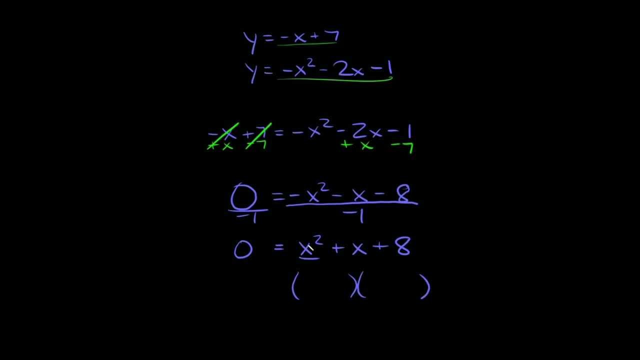 let's factor this: Okay, so here we have an x squared, So again we can break that into x times x, and then we have a positive eight here, right? So what two numbers can I multiply together to get positive eight? but they have to have a difference of basically a positive one, right here. right, the 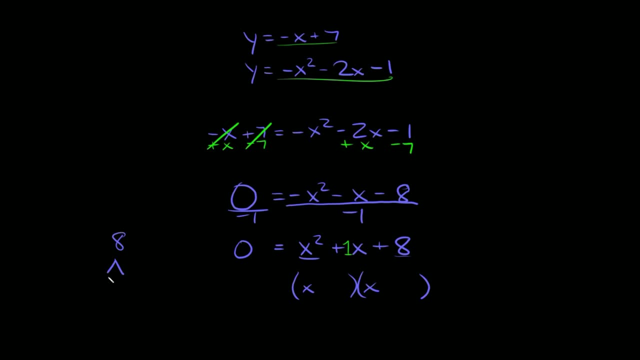 middle number. Well, in this case there is no solution, right, because the only ways we can multiply two numbers to get eight would be one times eight and two times four, right? So do either of these have a difference or do they add up to? I should say to positive one. No, because one. 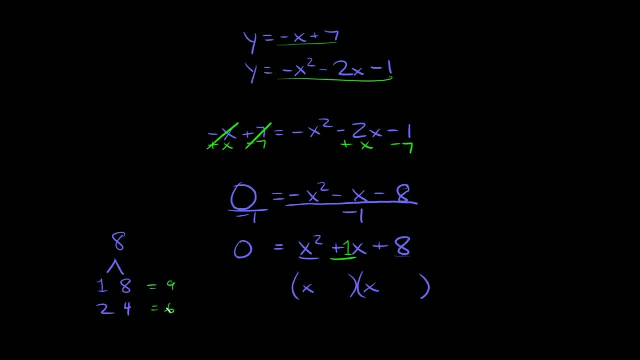 plus eight is equal to nine, and two plus four is equal to six, right? So neither of these pairs have a difference of positive one. So that means we can't actually factor this. Okay, and since we can't factor it, it's not factorable. that means there is no solution for this problem. So if you 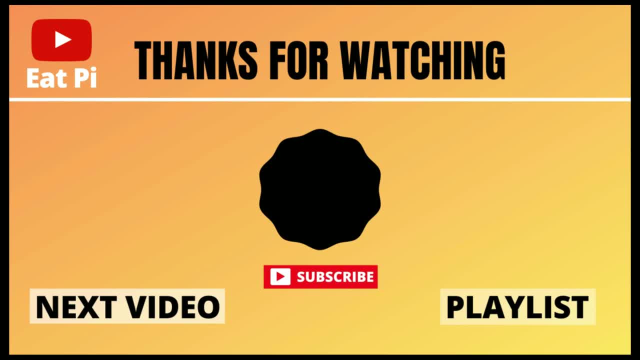 found the video helpful. definitely leave a thumbs up down below and if you have any other questions or want to see any other examples, just let me know in the comment section below.